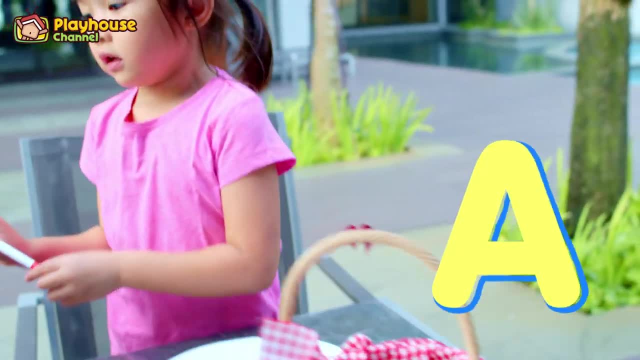 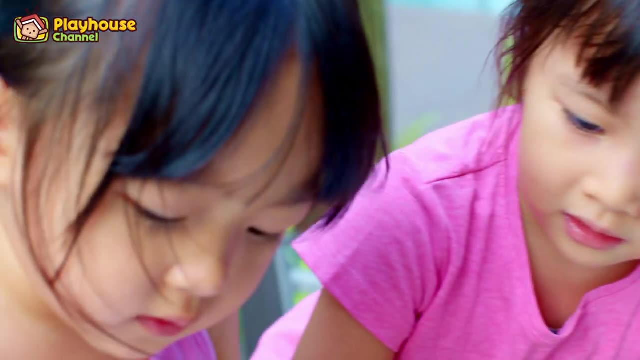 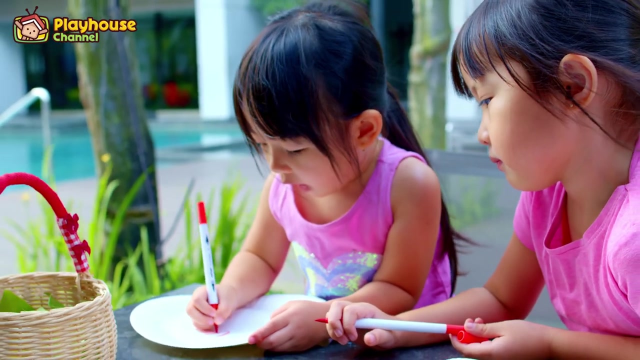 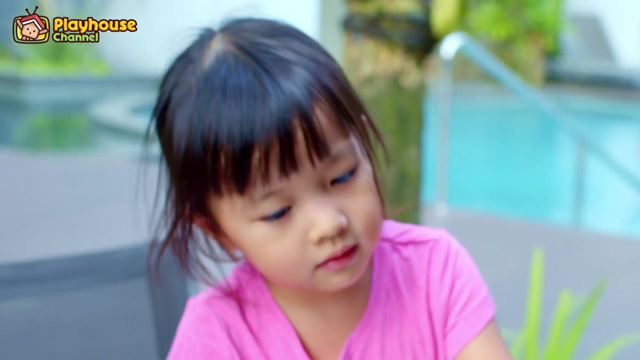 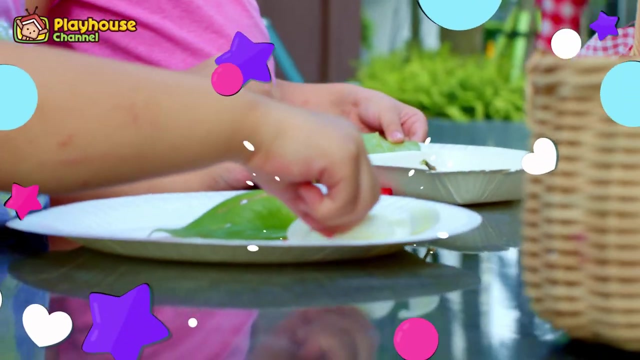 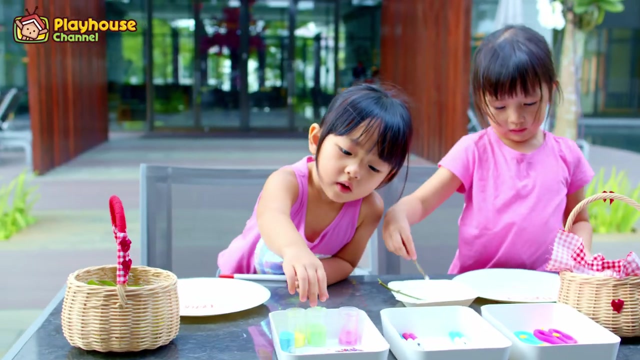 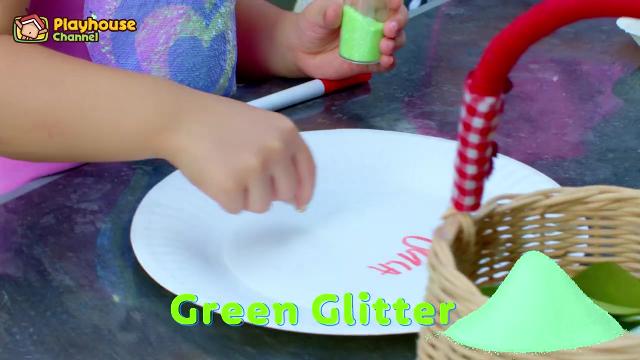 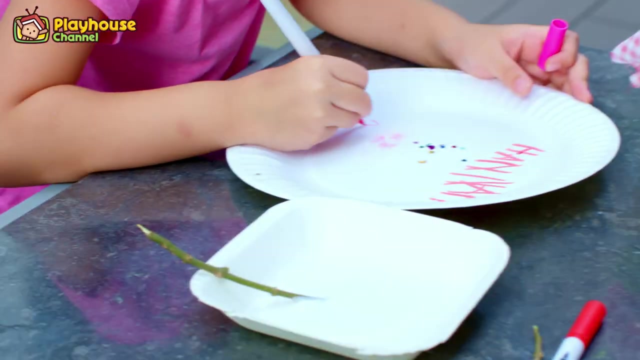 Oh, look, Look, Look. Now I'm gonna line it with my glitter paint. Now I'm gonna put back. Now I'm gonna line it again. I'm gonna use green glitter. Now I want to do some color pink to write my name, to write my mommy. 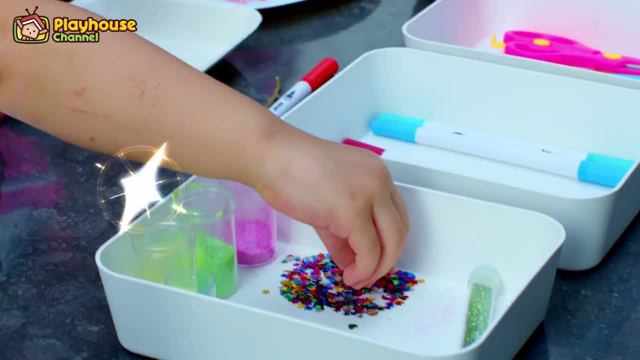 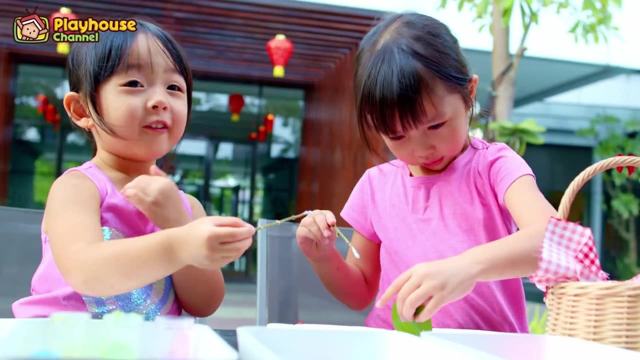 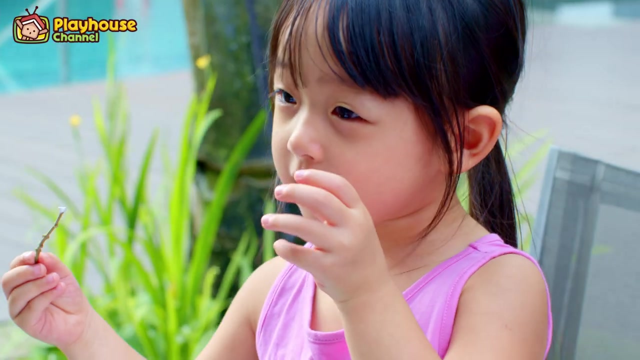 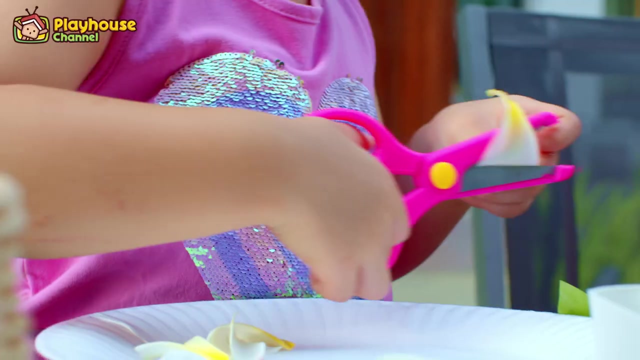 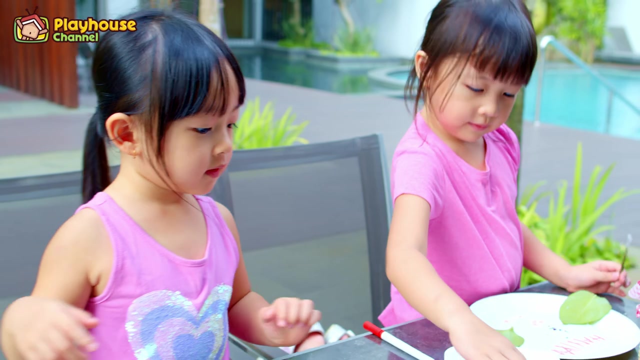 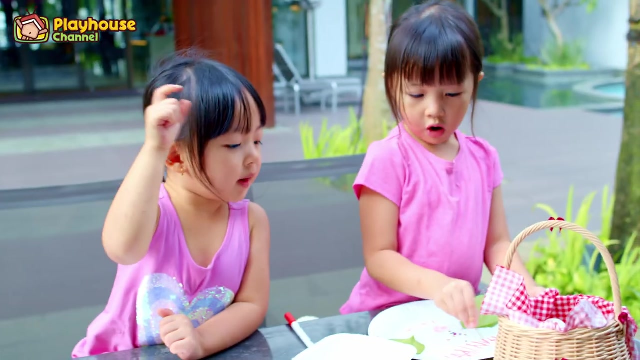 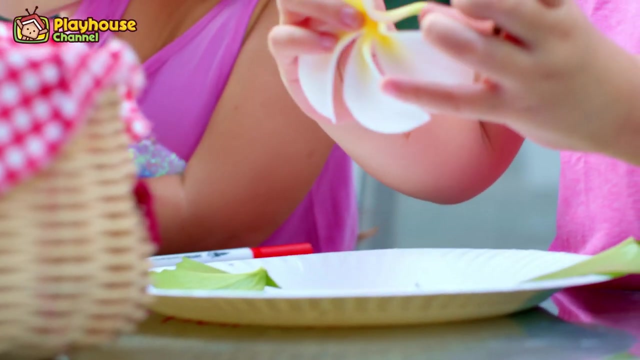 and now I put this. This is so much fun. Last time we made something with our mommy and it did like this. Now we put some flowers- Me too, I love flowers- Now, with my, with my, with my- I don't know You who didn't like doing. 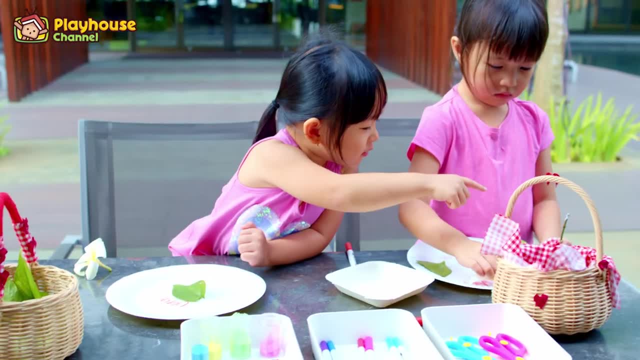 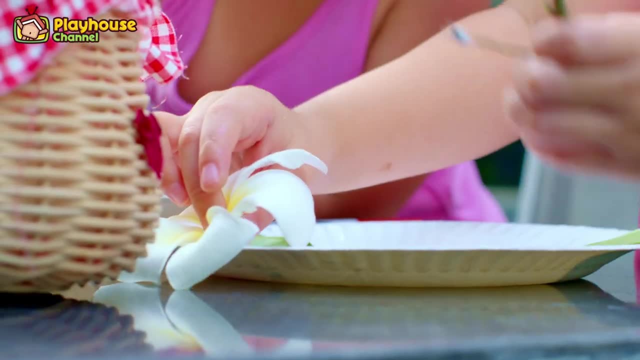 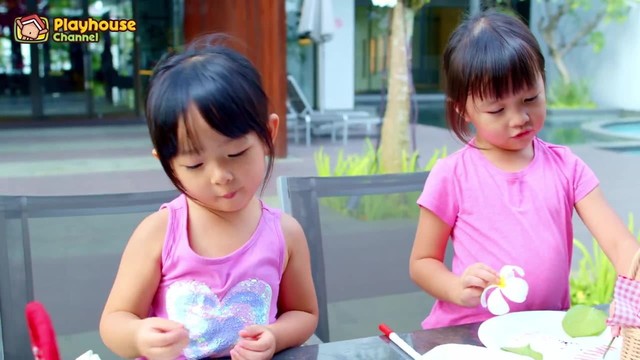 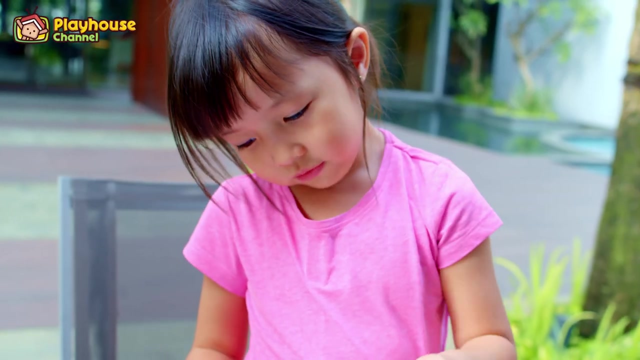 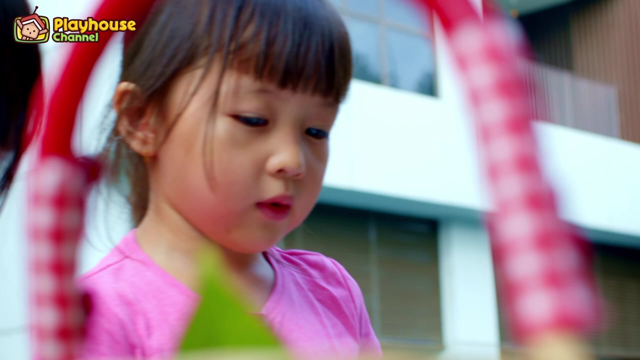 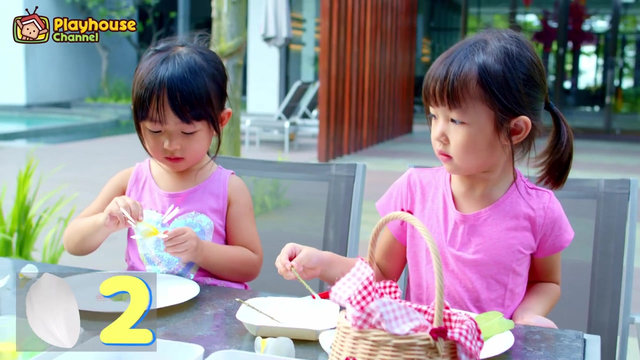 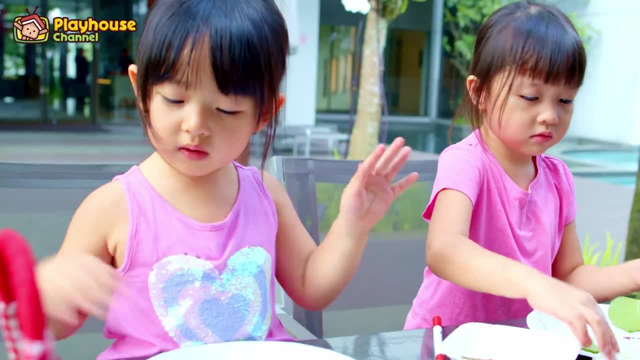 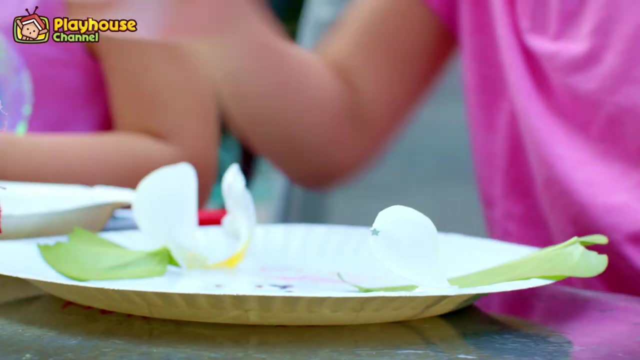 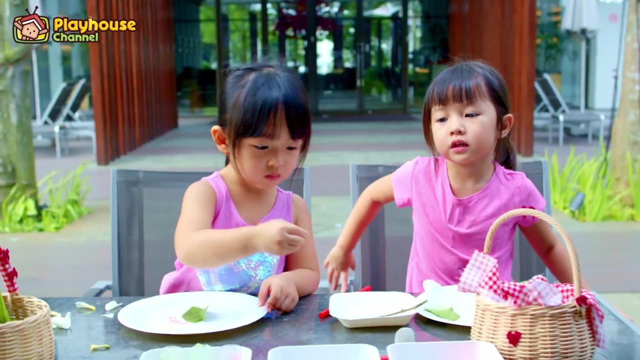 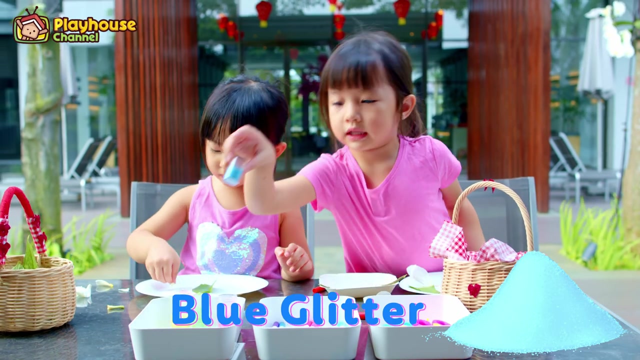 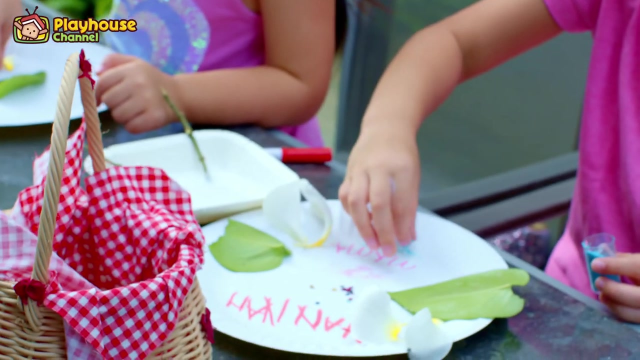 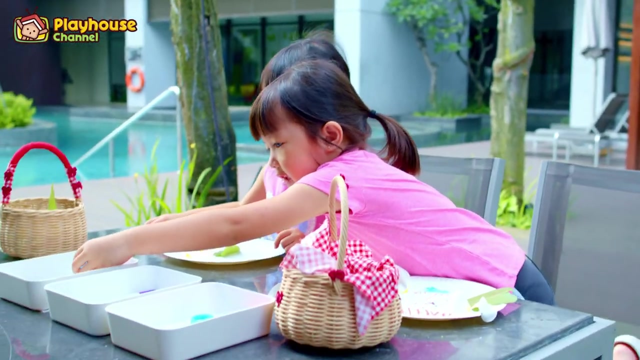 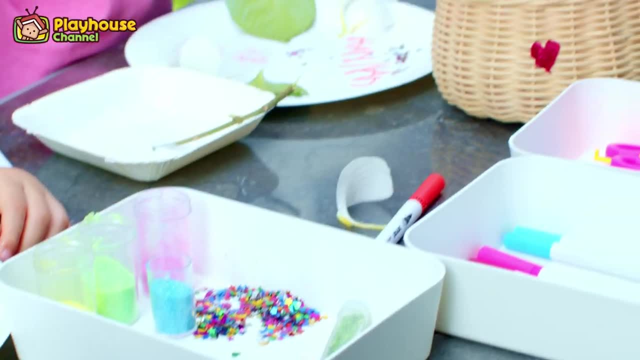 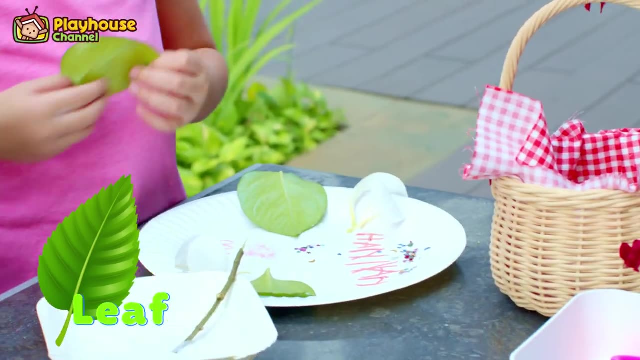 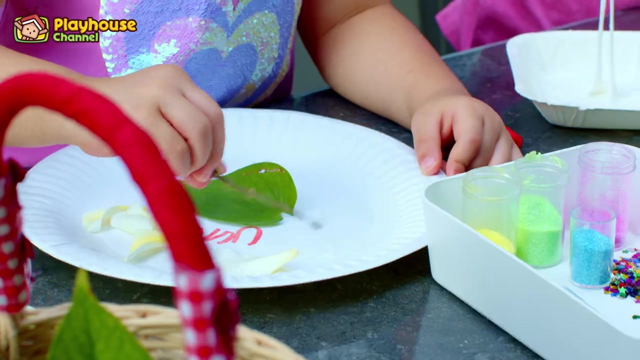 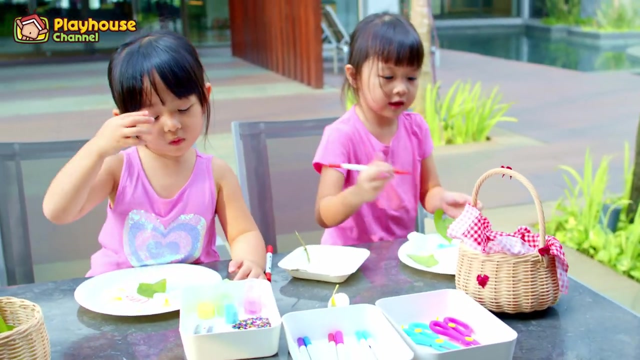 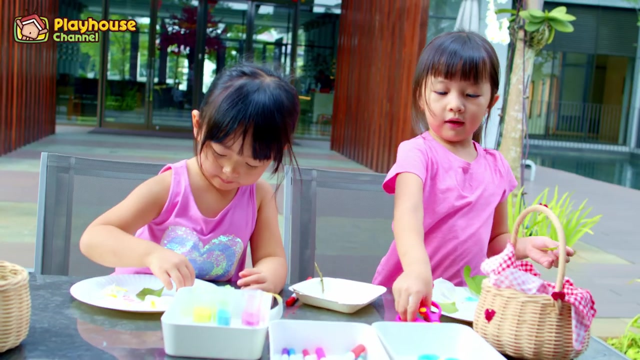 but we need lamp. Now I have to put a leaf on top, So I have to do like this, so I have to lamp it first. Woo This like stretch up. Now I'm gonna just write Jasmine, a sign on my name, chat zero. We have to lamp it. 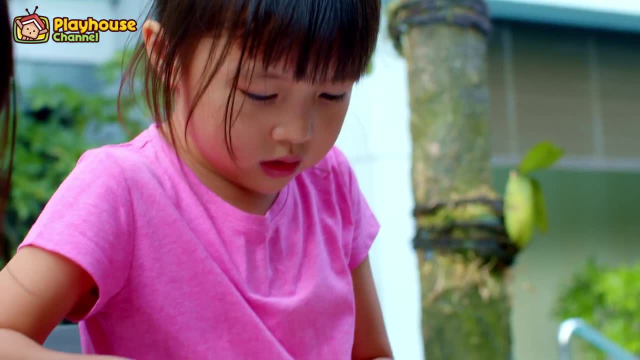 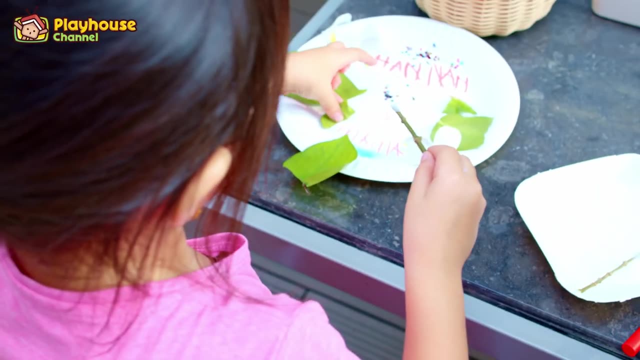 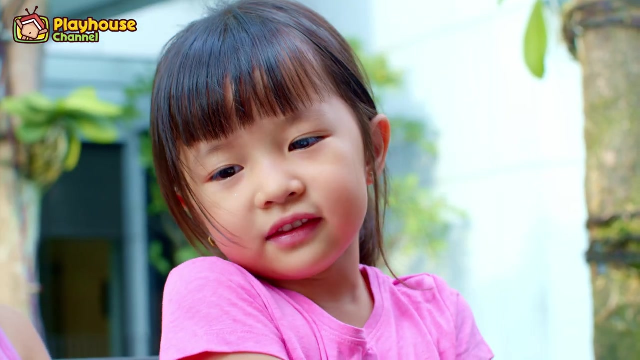 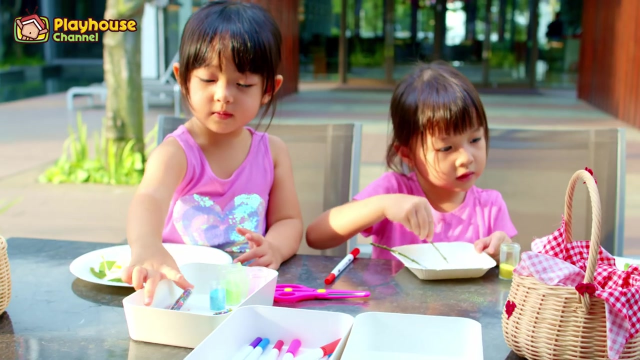 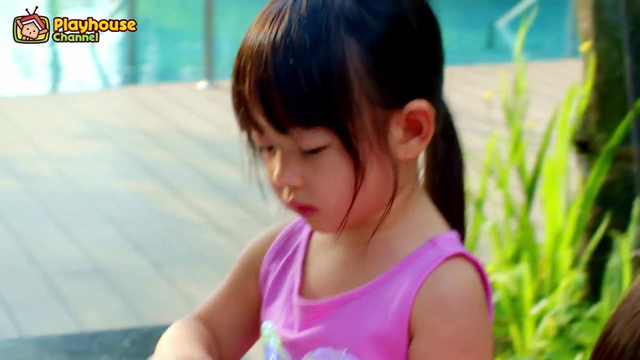 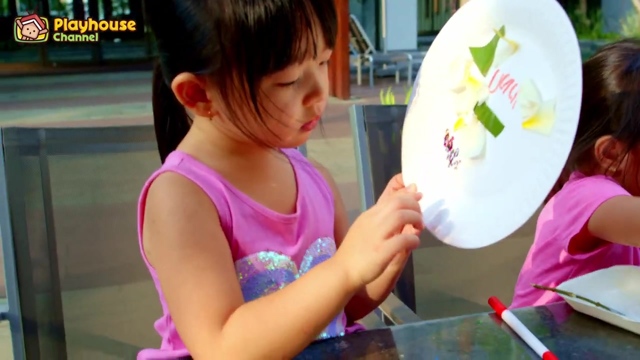 first, Stretch up Now, let's paste it. check Now. that's much better. Alana, are you done? Almost, I'm gonna put, I'm gonna. I'm gonna just put right here: I'm done, I'm not done. Okay, okay, I'm done, I'm not done, I'm so tired. 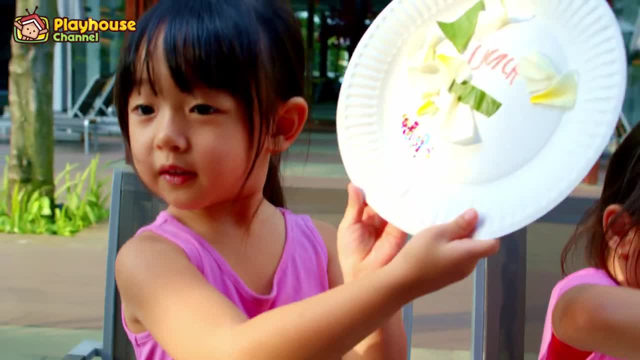 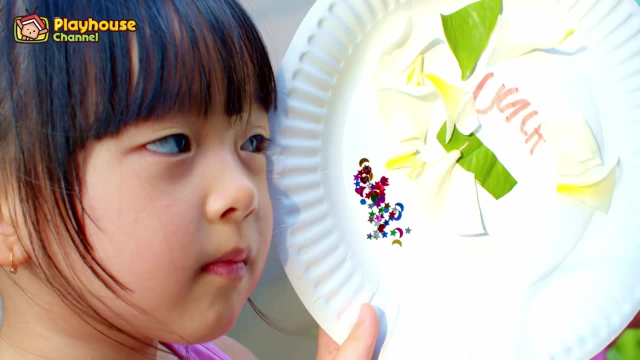 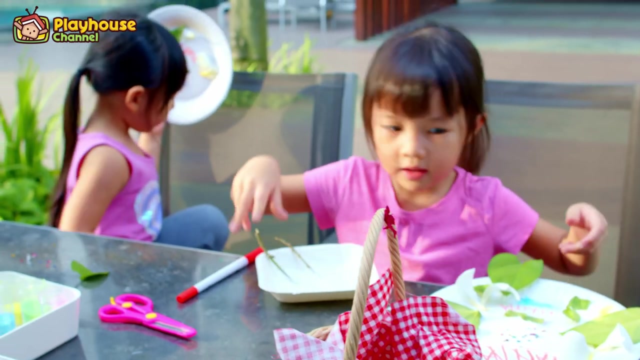 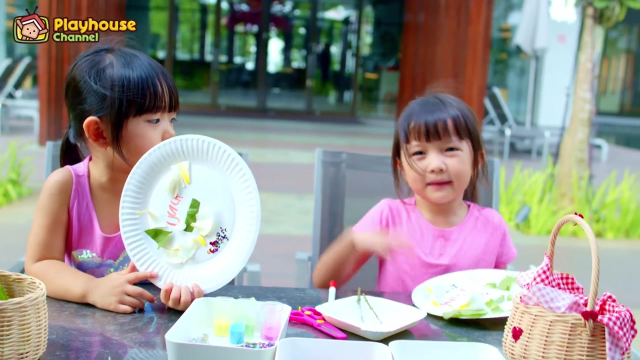 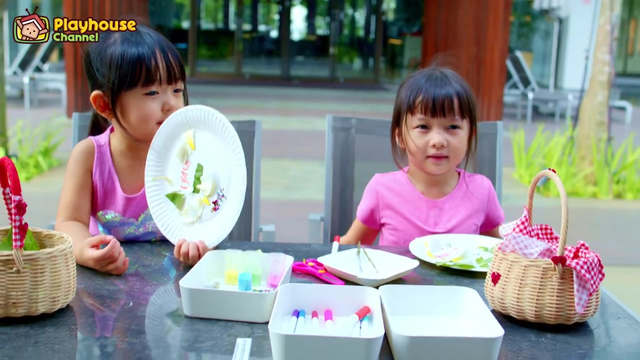 I'm done. Look at this, I'm not done. Alana, Just one more Just up here. I do it this way. There you go, bye, bye, Done. You cannot see, mom, Look at this, this is for my mommy, Bye. Thank you for watching Ni Hao's Channel. Ni Hao's Channel. Ni Hao's Channel.